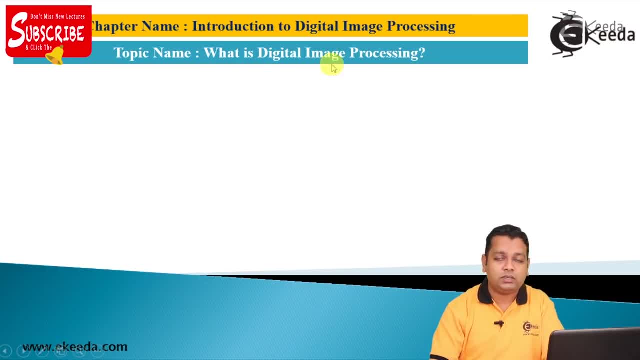 Those viewers who are very beginners with the subject digital image processing, I must make you familiar that we should first of all have the image That generally we obtain with the help of camera. in our subject We call this process as image acquisition, and the camera is actually the image sensor. 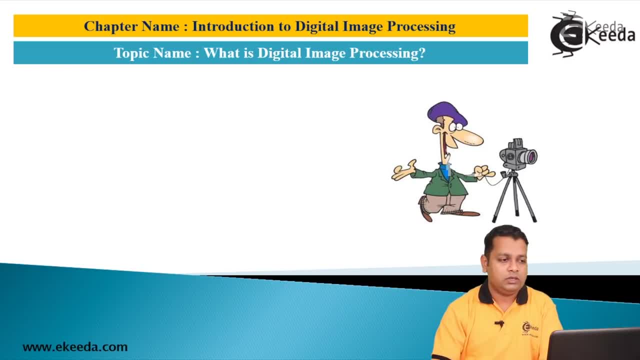 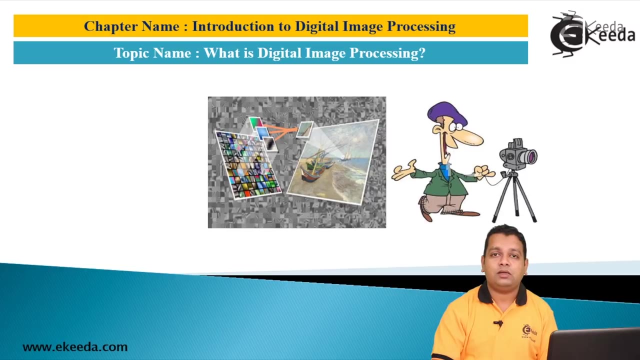 With which a picture generally what we term is our image, So that image should be digital image. That image contains information, So the extracting information from the digital image and processing it further for the specific application we can say it is the extent of digital image processing. so this is a try to show you a prototype of what exactly digital image. 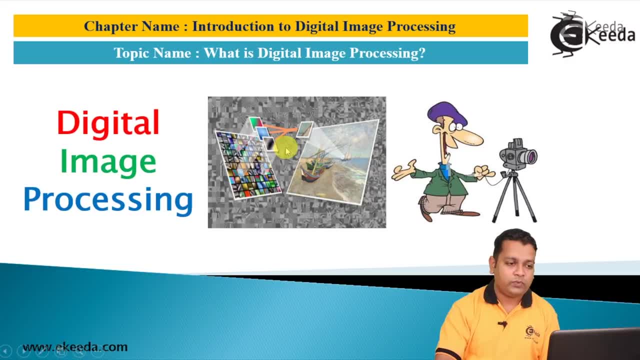 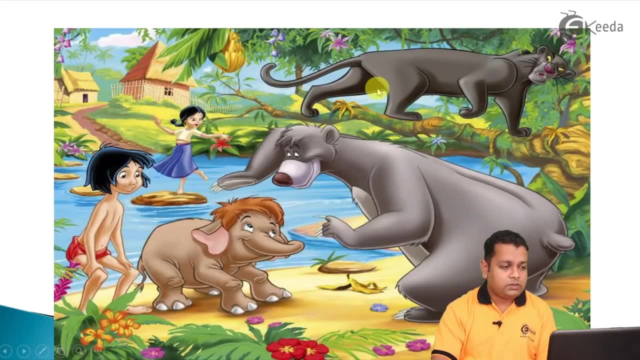 processing is: yes, the title is digital image processing. moving further into the topic, we first of all take a simple picture here. this picture contains a cartoon character, mogli, here, a dancing girl, a calf of elephant, uh, black bear, black panther. we have small huts here, the forestry. 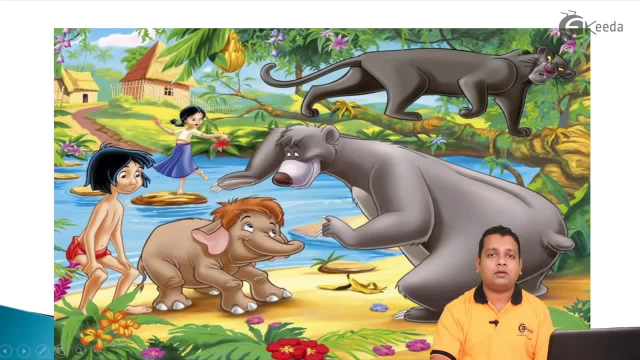 the river. a lot of things, along with the fruits, are there into this image. so lot of storytelling things can be done with the help of this particular picture, what we call image also hence. anonymous person has said that one picture is worth more than 10 000 words here. so with this, 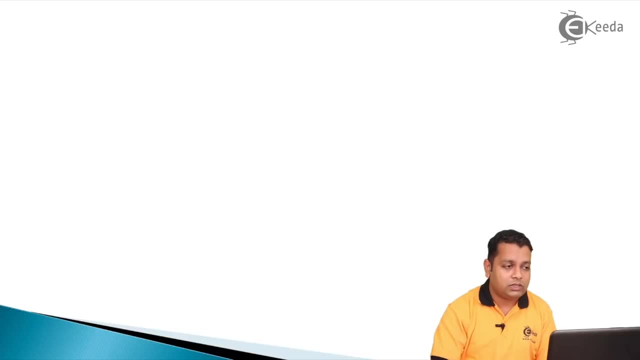 understanding. we begin with the topic: what is digital image processing? so let us first of all see what is the motivation behind the development and the popularity of digital image processing. it is mainly because of the two application areas, or the two causes, we can say, that are listed here. 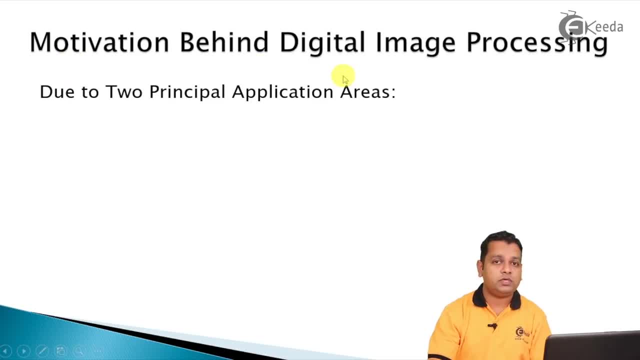 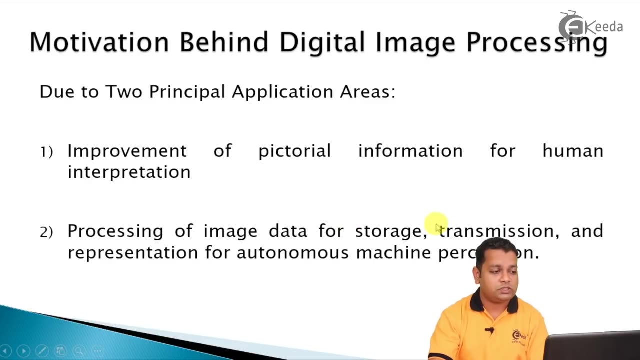 so here we can say that the motivation behind digital image processing is due to two principal application areas. the first one is improvement of pictorial information for human interpretation and the second one is processing of image data for storage, transmission and representation of autonomous machine perception. so here these two points are very much important. 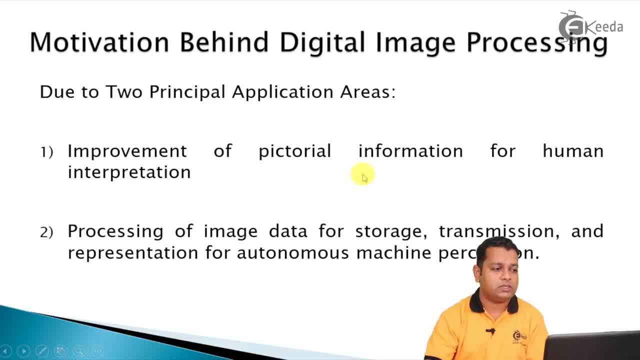 whatever the information we get from a certain image- that is addressed into the first point- we always want more information to be obtained. so, from the image we want the pictorial information to be improved, one for our interpretation- human interpretation, we can say- and when the task of storage of that particular information. 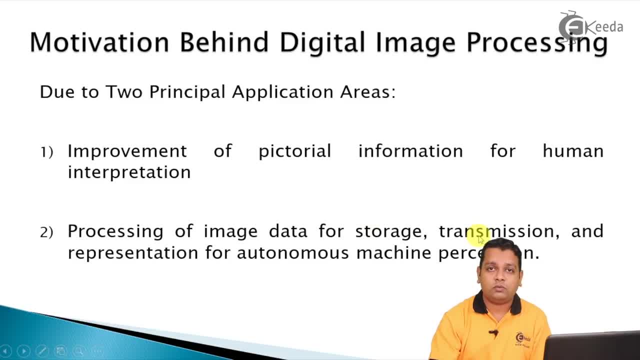 to reproduce it later on or to transmit that information from one place to another place, and representation onto the displays of the modern computers or the modern machines. we can say the second point is said that processing of image data for storage, transmission and representation of autonomous machine perception. so these are the two causes because of which the high development. 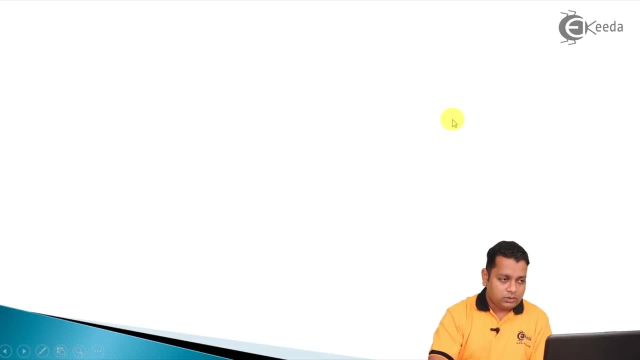 into the digital image processing has taken up further. we shall see the three terms for the subject that is digital image processing. and here, out of these three terms, we first of all begin with the middle term, that is, what exactly the image is. then we shall see what exactly the digital 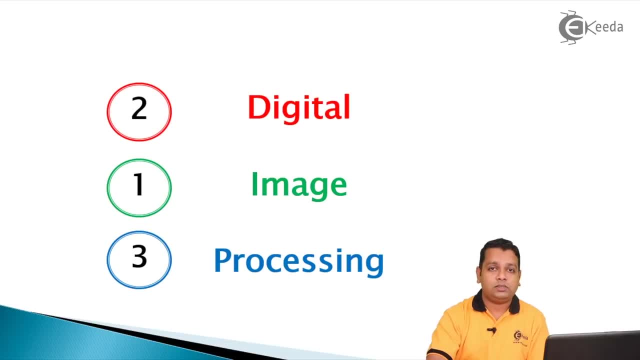 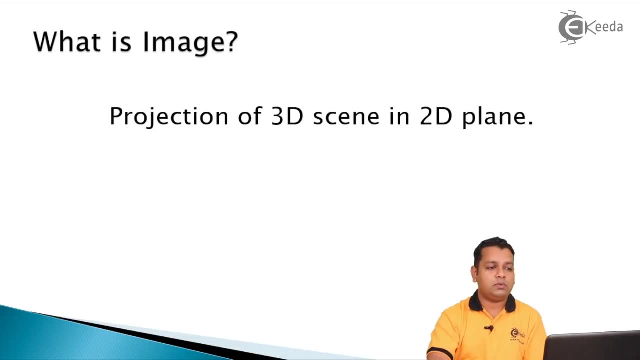 image is, and then, lastly, we can see the digital image processing. so, very first of all, the question is: what is image here? so, regarding the image, we can say that it is the projection of 3d scene into the 2d plane. whatever we see with our bare eyes, that is actually. 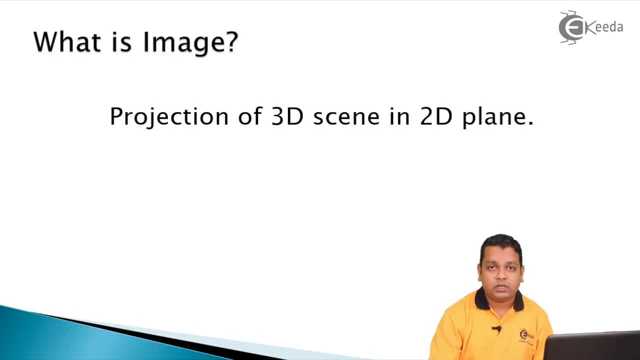 a three-dimensional view that we can model with the help of three axis XYZ, that we have to do the representation onto it 2d plane or a plane of paper. we can say so here: the three axis XYZ, the 3d scene, we have to model in terms of only the two axis. that exactly means the image. so here, 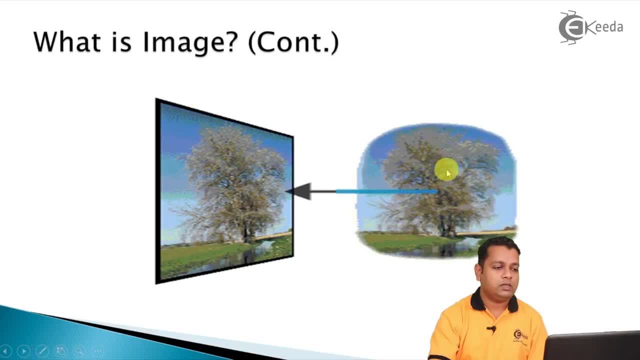 the example with this, with the help of this picture, we can see- so this is a tree- into the three-dimensional view or three-dimensional scene. we can see that we have captured an image into the two-dimensional plane here. so this is the general interpretation of what exactly the 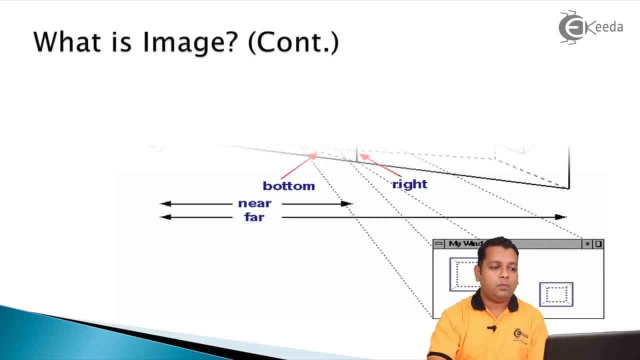 image is now talking further. we can have a simple model here, as the natural source of capturing image is our eye. so here we can have into the scenario the two objects. into this diagram you can see that the two objects are of same dimensions, but they are located apart from each other, so the 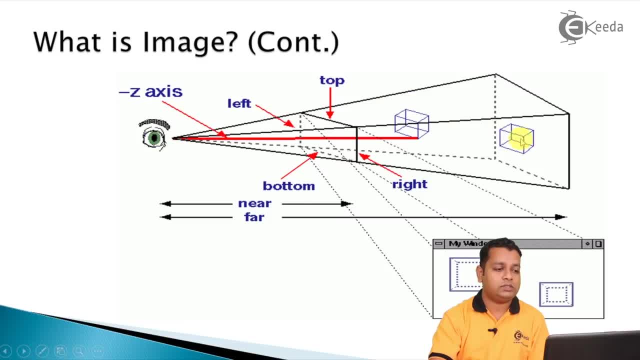 first object is near to the eye, the second object is far from the eye. so, whatever the image that generally we say is formed onto the retina, that will be a two-dimensional image for our interpretation, and here, though, the two objects are of same dimensions. the object that 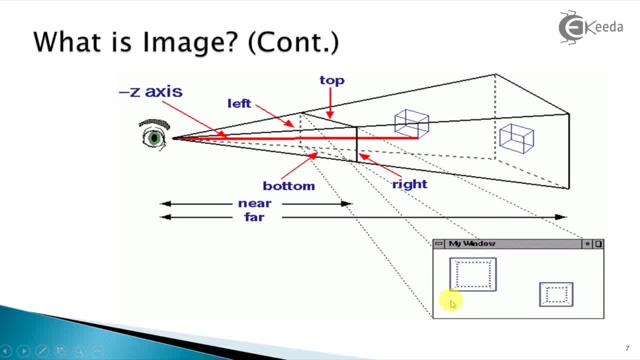 is near to eye, that is having the higher dimensions into the image, and that is far away from the eye, that is having the smaller dimensions into the two-dimensional view here. so the 3d scene, that exactly, is the image here. further we can say that mathematically talking, we can have the definition. 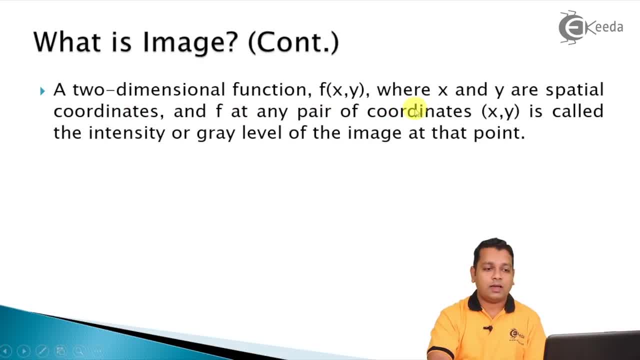 a two-dimensional function, f of x- y, where x and y are the spatial coordinates, and f at any pair of coordinates of x- y is called intensity or a gray level of the image at that point. so here we can take the two axes, x and y. so x and y will give the spatial coordinates the location of the. 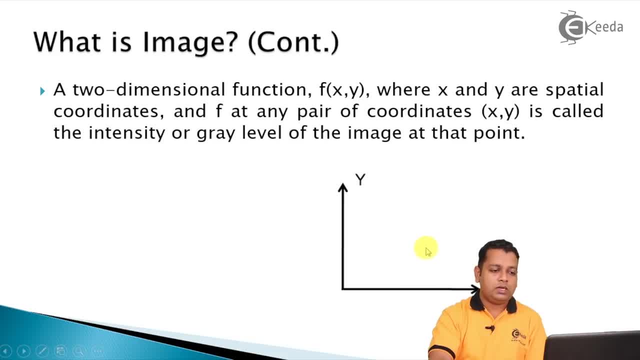 elements of this particular image, so defining the exact values of x and y at that particular location. there is third parameter, that is f, which shall give us the intensity of the gray level of the image at that particular point. so, depending on the x, y and f values, we can have the classification. 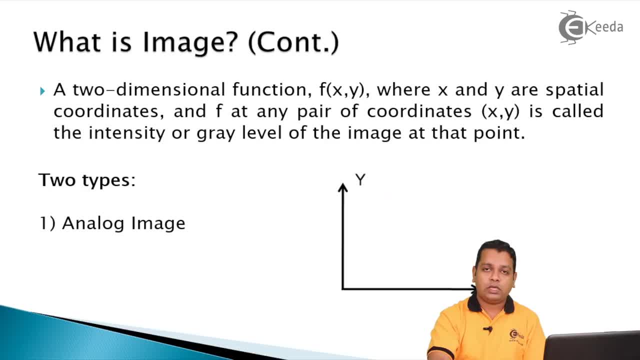 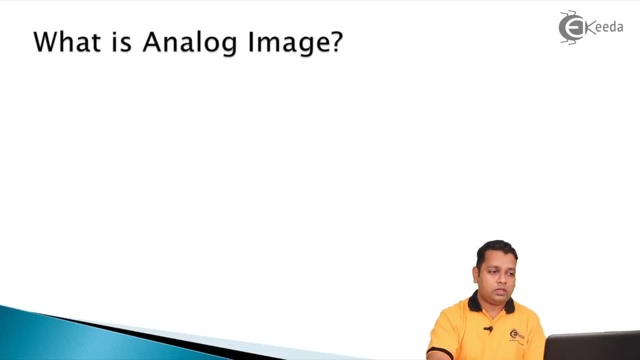 of image into the two types, that is analog image and, what is our important one, that is digital image. so let us first of all talk about what exactly? the analog images, then later on we shall see the digital image. so for analog image, first of all the accepted definition, for simply the image. 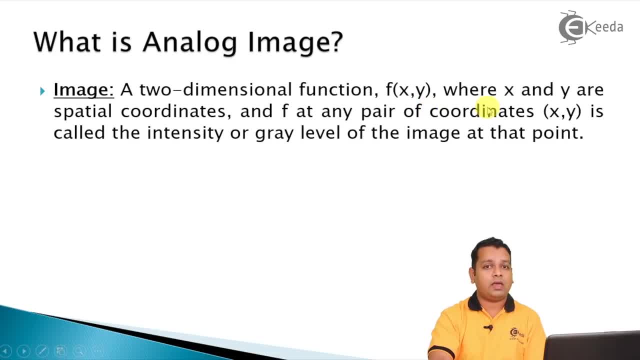 is a two-dimensional function: f of x- y, where x and y are the spatial coordinates and f at any pair of coordinates. xy is called the intensity or gray level of the image at that particular point. so the an radish for the image to be analog image is that when these representations has the continuous range. 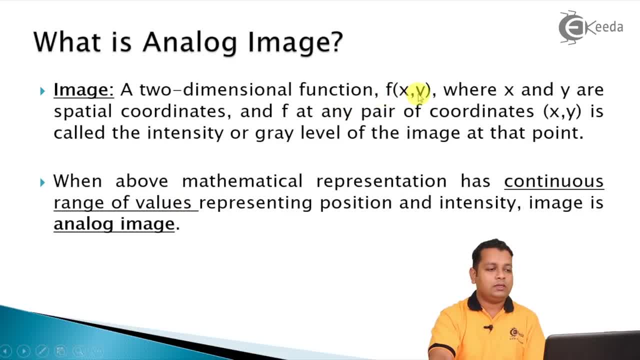 of values for f, x and y, representing the position by x, y and the intensity by the parameter f, so that time we can say that the image is analog image. The example of analog image can be given as the image produced onto the screen of CRT. 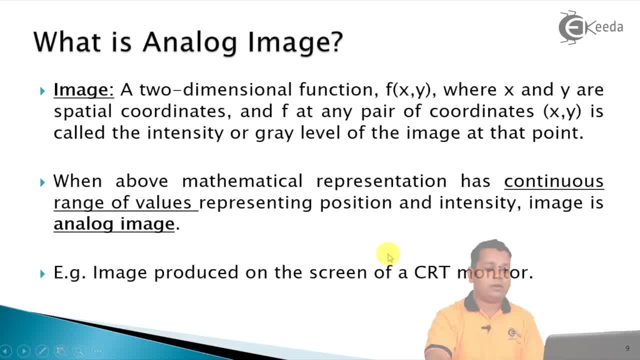 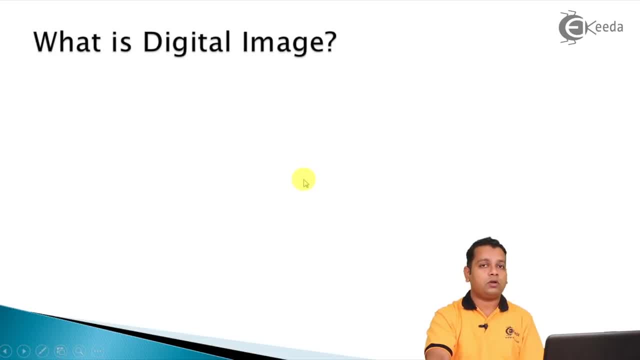 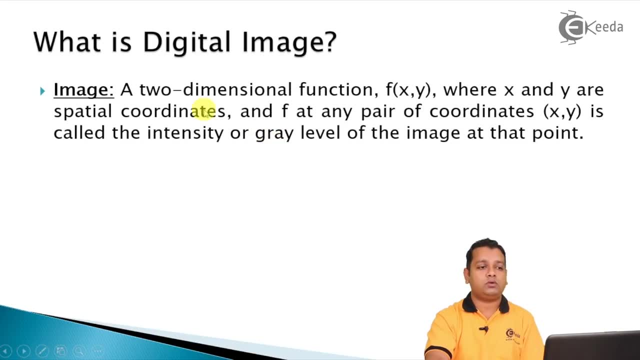 monitor. The storage requirement for such analog image is having the high memory. Further, we can talk about the digital image, which is of more concern to this particular subject: digital image processing. So again we have the accepted definition of image into the mathematical form. It is a function, f of x, y, x, y being the spatial coordinates and f is the intensity. 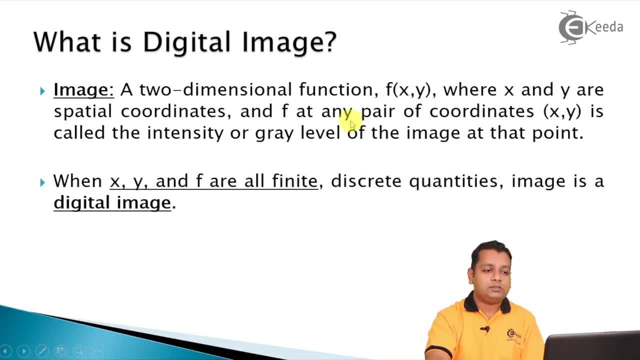 or the gray level of the image. So when these three parameters are discrete into the nature, All x, y and f, in other words we can say, are all the finite quantities. that time we can say that the image is a digital image. So just now we have seen the two types of images basically, that is analog image and 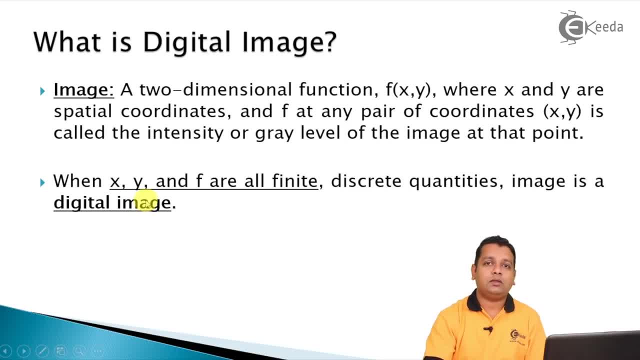 that of digital image. So generally in our world we have the analog everything, but for the storage purpose, for the transmission purpose, we convert it to the digital domain with the help of digital computers. So we have to obtain a digital image from the analog image. 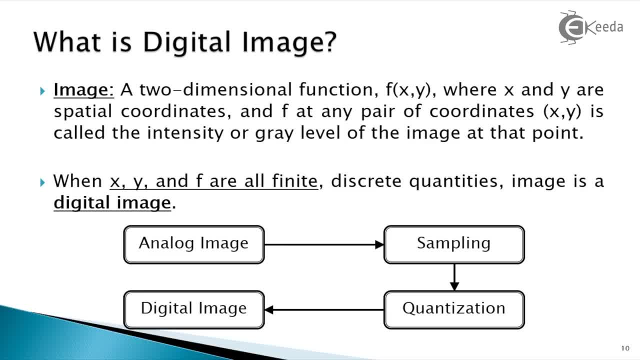 So for that purpose, this simple procedure is to be obtained from the analog image, We have to do the sampling, and the sampling will have the discretization in terms of x and y. after sampling we have quantization, which will have the discretization onto the f parameter. and after sampling and quantization, we obtain the form of image to be the digital. 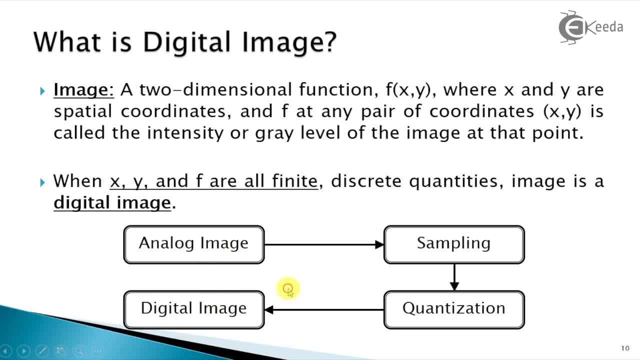 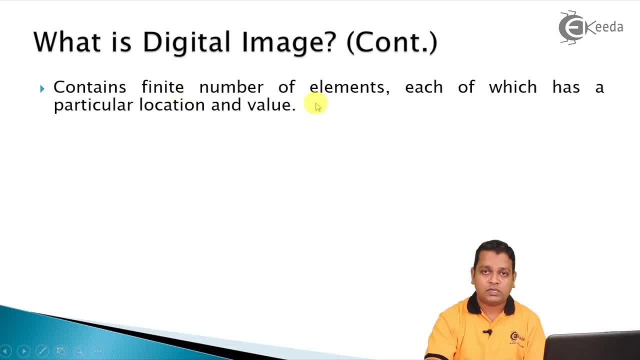 image. So this is exactly the digital image is So more information. regarding digital image. we can say that it contains finite number of elements, as all the three parameters, x, y and f, are all discretized here. So these number of elements, given with the discrete values of x and y, we can say each. 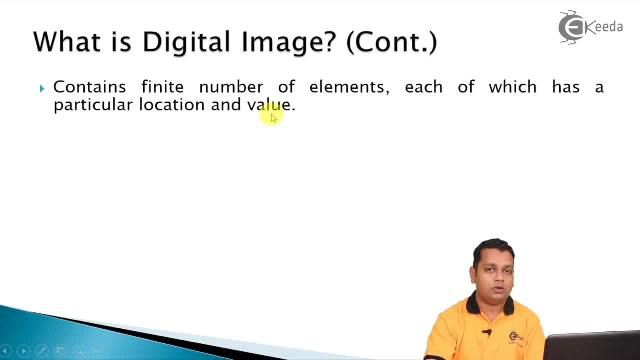 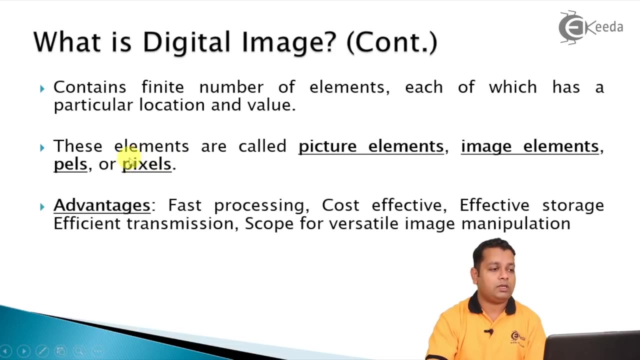 is having a particular location and a certain value of f here. further, such elements we can call the picture elements, also called as image elements, PELs or pixels. Pixel is the most widely term that is used for representation of such elements into the digital image. 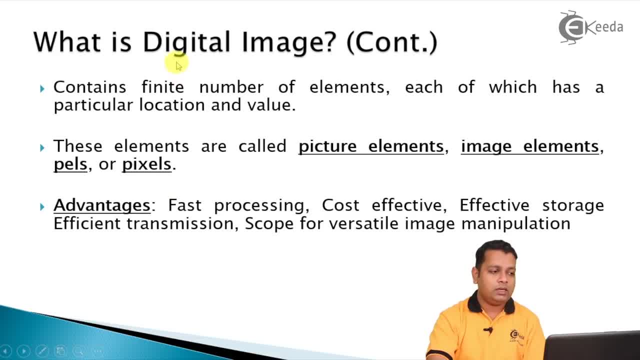 So what are the advantages of having such a digital image? The advantage is that fast processing, as the memory requirement is less as compared to the analog image, It is cost effective. It has effective storage, effective transmission from one place to another. It is cost effective. 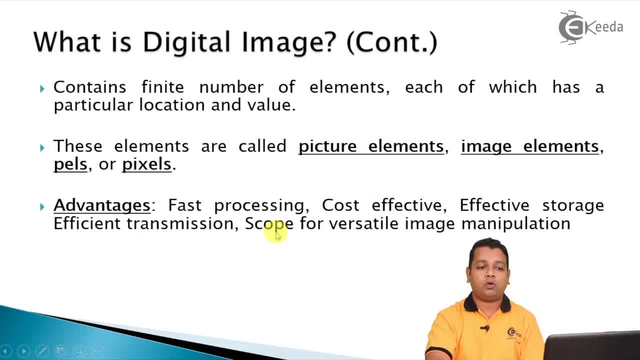 It is cost effective, It has effective storage, effective transmission from one place to another, along with the scope for versatile image manipulation. Image manipulations we can do with the digital image. So what are the disadvantages? The disadvantages is that high memory is required if you want the good quality of images and 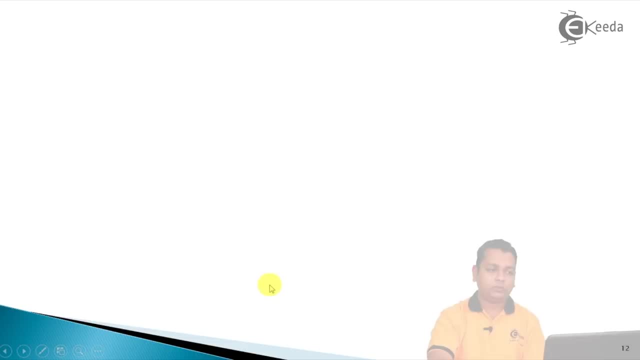 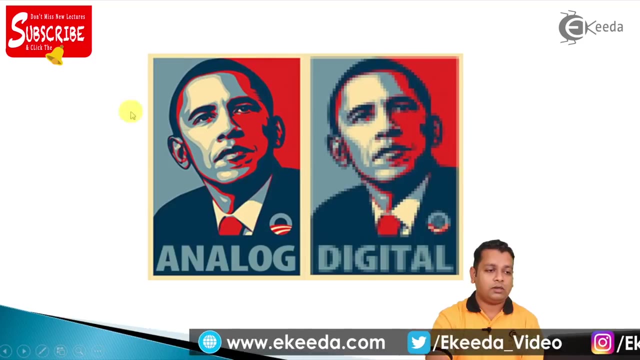 hence requires the fast processes here. Further, if you like to compare the analog image and the digital image, here we have a sample picture here. first image is having a very precise curvatures, the edges we can see. hence the storage of this particular image requires higher memory. this image can be said to be the analog, here all the x, y and 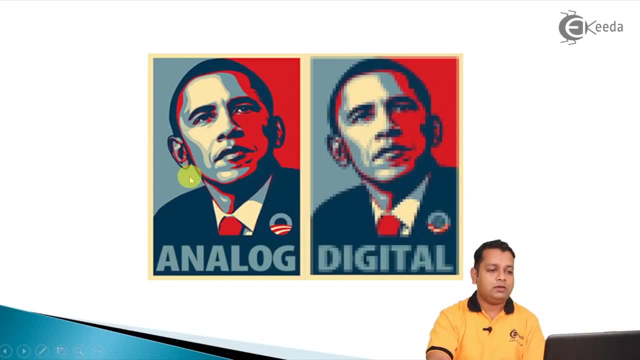 f value are continuous here, whereas into this second part, that is said to be the digital one, the things of x, y and f are discretized here. they are not the continuous range of values for x, y and f. that is the basic difference between the analog and the digital image. now further. 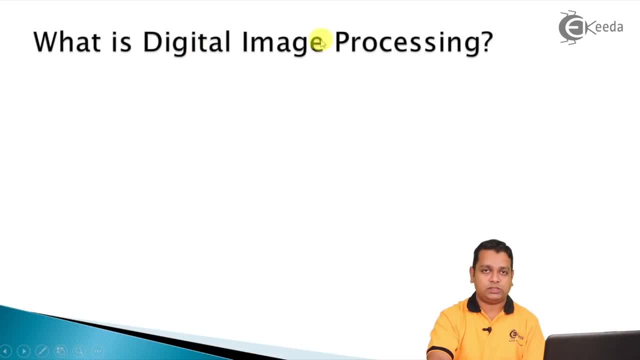 we shall see what exactly the digital image processing is. up till now we have seen what exactly the digital image mean, so we shall see the processing. so into a single line, we can say that the analysis and manipulation of the digitized image, especially in order to improve its quality. 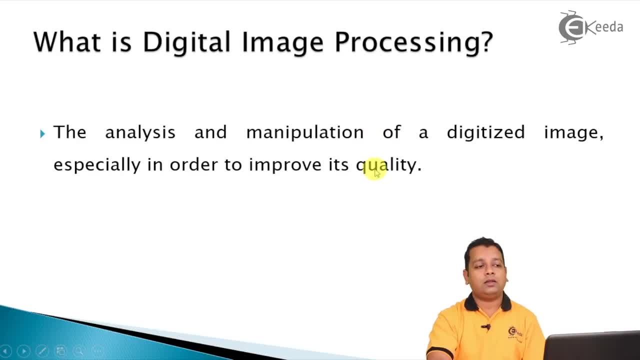 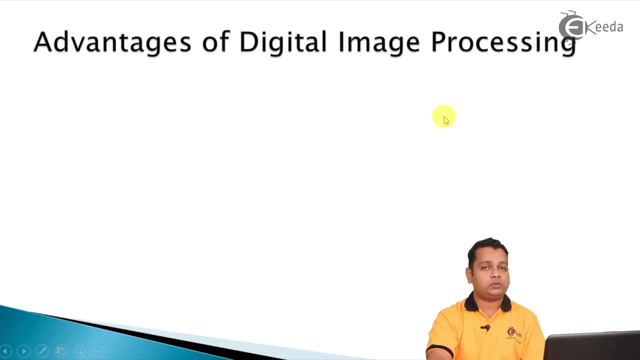 is said to be the digital image processing. in another words, we can say that processing of digital images by mean swap digital computer for specific applications is actually the digital digital image processing here now, what are the advantages offered by the digital image processing? the advantages offered are, as we know, the human beings all of us are. 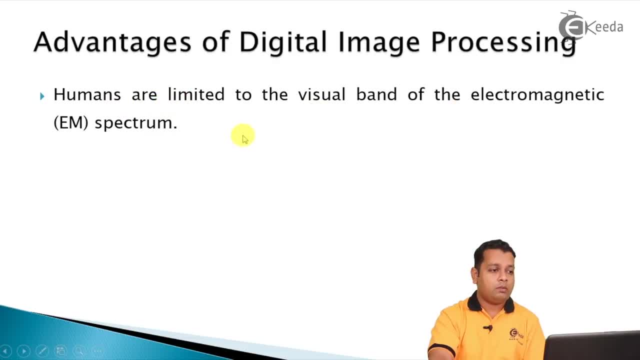 limited to the visual band of electromagnetic spectrum. but as we talk about the storage, transmission with the help of machines exactly can see or the digital computers, so the imaging machines cover almost the entire EM spectrum, ranging from gamma waves to the radio waves. as we are confined to only the visual band, the machines 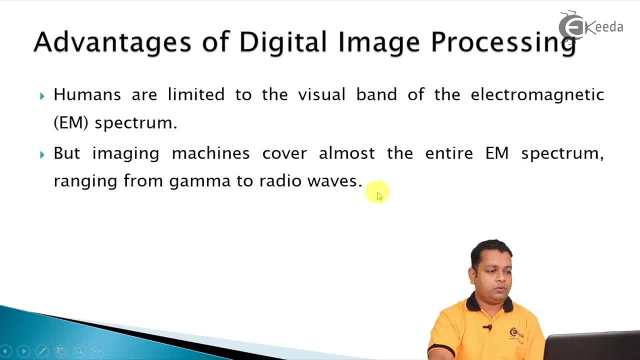 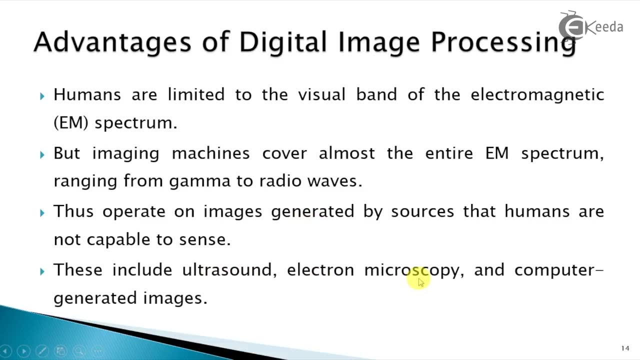 can cover the entire electromagnetic spectrum so further, thus operating onto the images generated by sources that humans are not capable to sense we can have into the digital image processing. so these include ultrasound electron microscopy and computer generated image. hence I can conclude that the advantage of using digital image processing is to have more information that 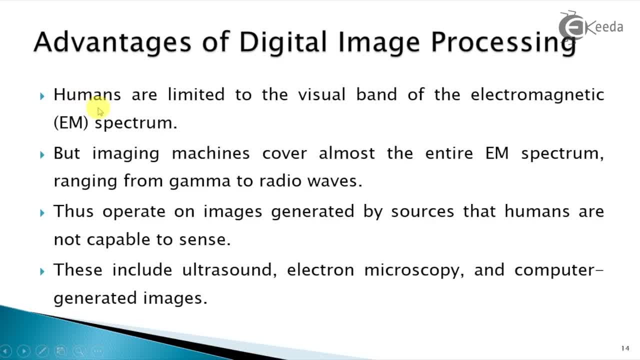 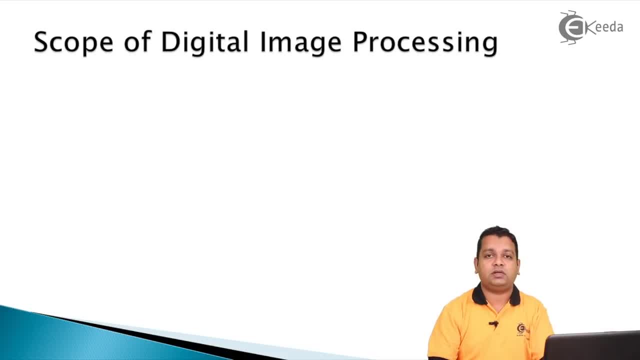 only the human beings directly are not related to. so, after advantages of digital image processing, let us address what is the exact scope of digital image processing. the very first point we can say here that there is no general nature of digital image processing and it is not exclusive to. 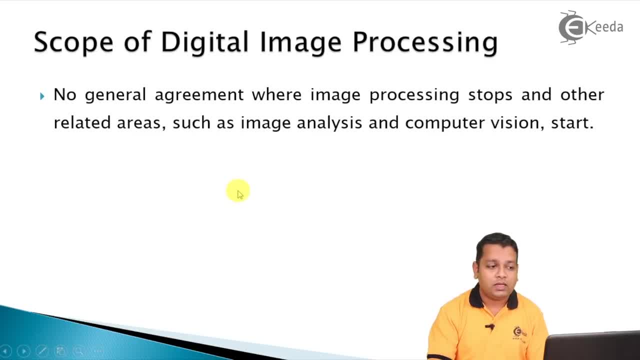 digital image processing. but we can say that there is no general nature of digital visual images, general agreement where the image processing exactly stops and the other related areas, such as the image analysis, the computer vision, start here. Along with this, the distinction sometimes for digital image processing is made that 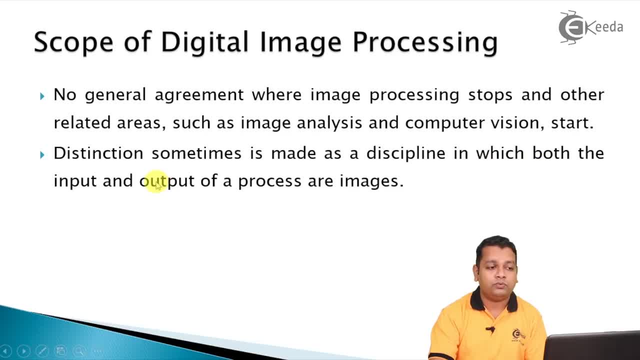 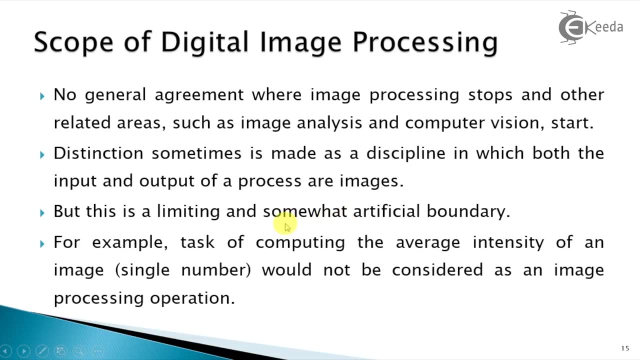 it is defined as a discipline in which both the input and output of the process are the images here. But this definition is sometimes limiting and somewhat artificial boundary for that purpose. We have the simple example here: if the task of computing the average intensity of an image 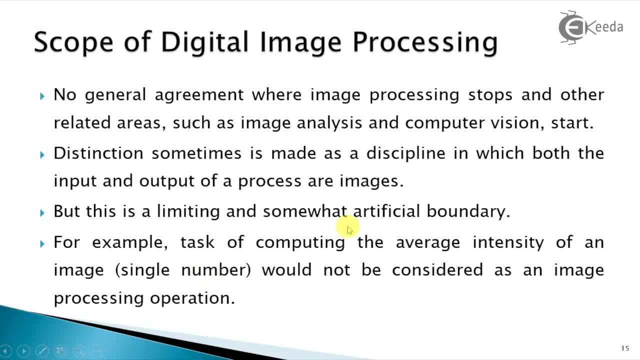 which is exactly a single number. So according to this definition would not be considered as image processing operation, But we know that it is a task that is associated into the digital image processing only. So there is No general agreement and no general definition where we can exactly say the scope of digital 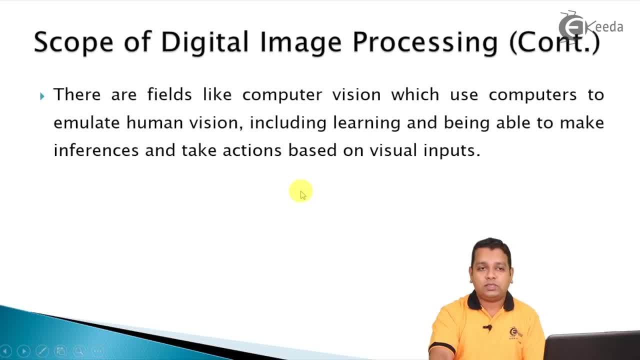 image processing is defined here. So further we can say that there are the fields like computer vision, which use the computers to emulate the human vision, including the learning and being made able to make the inferences and take the actions based on to the visual inputs. here does a branch of artificial 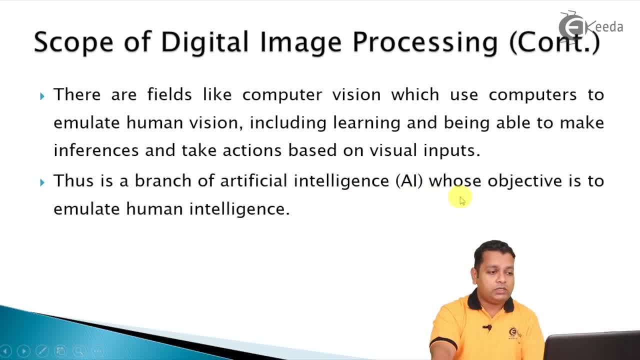 intelligence. AI- This is an abbreviate whose objective is to emulate the human intelligence- is here, It is the computer vision and hence the area of image analysis along with these understandings. We can say image understanding for the image analysis. Also, it is in between the image processing and computer vision. 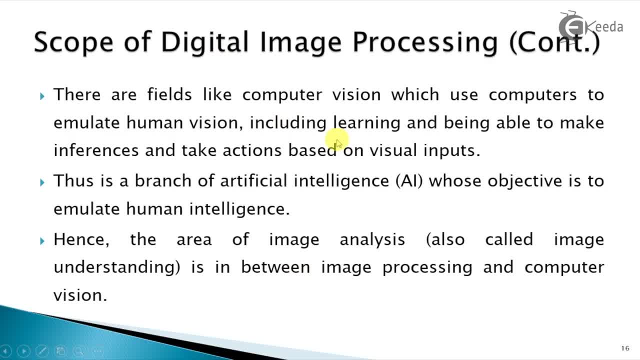 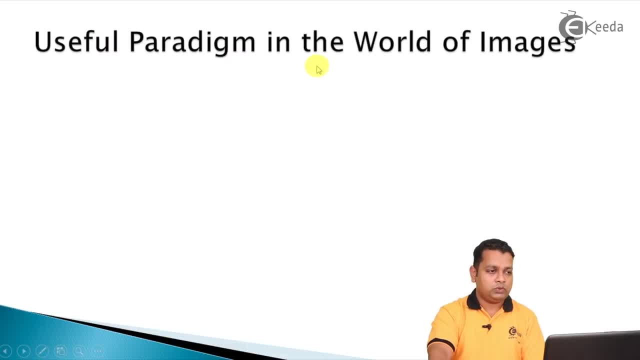 So, as the digital image processing, the start and end lines are not clear cut, We have a paradigm which is useful in the world Of images. so useful paradigm in the world of images, We can see that consideration of the three types of computerized processes. 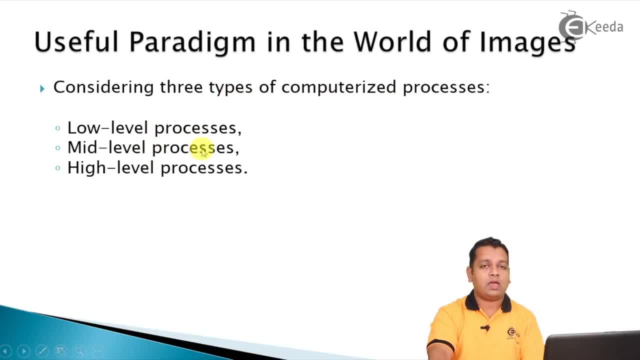 We can say low-level processes, mid-level processes and finally the high-level processes. talking about the first process, that is, the low-level process, We can say that this involves primitive operations such as image pre-processing to reduce the noise, to have the contrast enhancement and to have image sharpening. 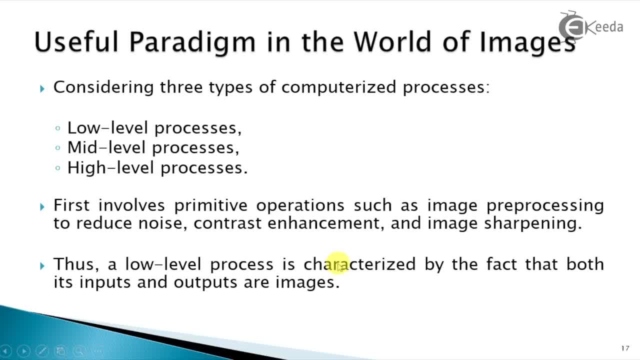 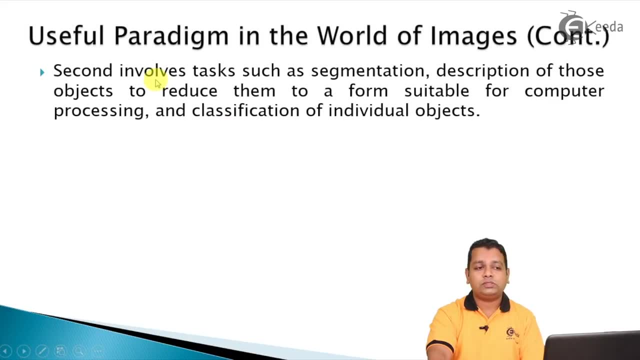 So further, this low-level process is actually characterized by the fact that both the inputs and outputs are the images. So this, we can say, is exactly the low-level process. further, talking about the mid-level process, We can say that it involves the task, such as image segmentation, that we are going to 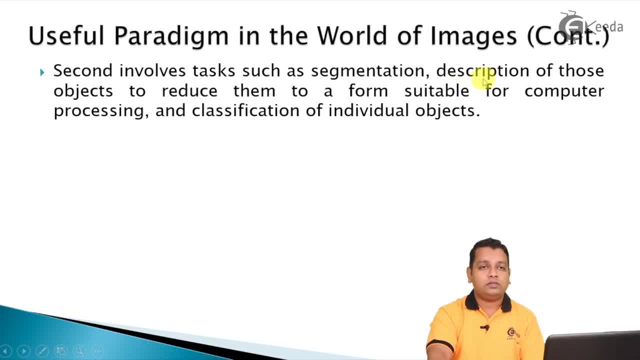 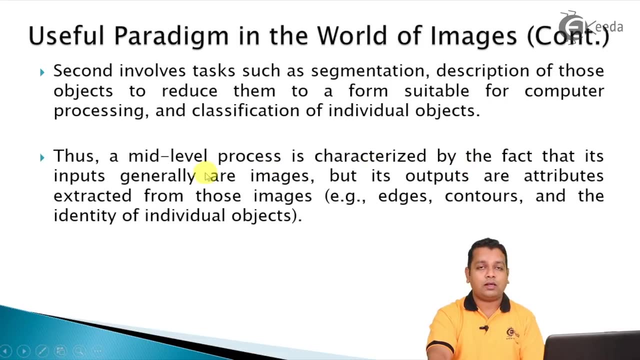 see into the details, into the next chapters, Definitely the description of those objects to reduce them to a form suitable for computer processing and classification of individual objects. So the mid-level process is characterized by the fact that its inputs are generally the images but the outputs are actually the attributes extracted from these images. 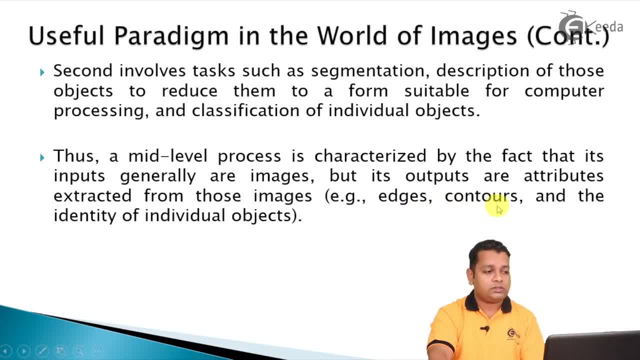 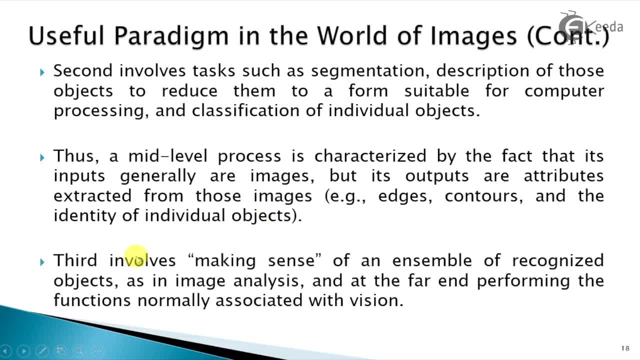 The attributes are in the form of edges, counters and the identity of the individual objects. here, Finally, the last one, that is the third, that is, high-level process, according to this useful paradigm, It involves making sense of the ensemble of the recognized objects, as in the image analysis. 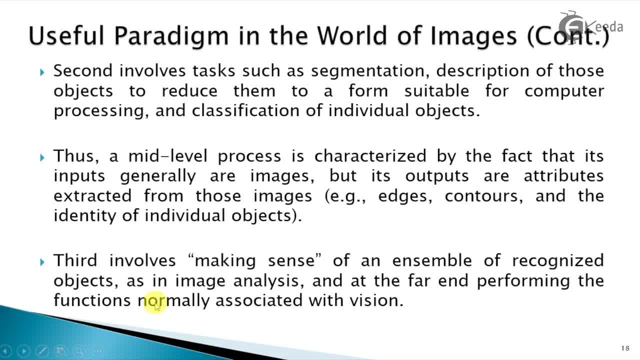 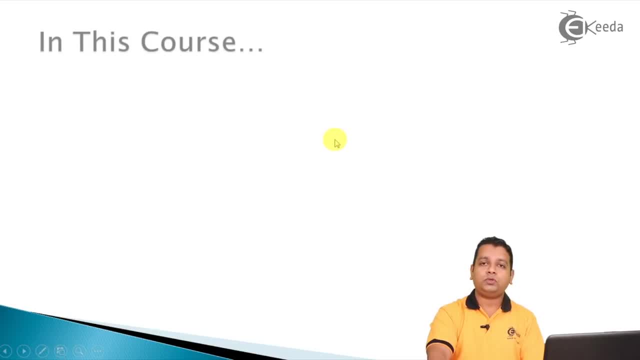 and, at the far end, performing the functions normally associated with the vision. Hence by the title useful paradigm in the world of images, we can address right from the digital image processing to image analysis and finally the computer vision. So in this course into the digital image processing, we are going to address first of all the first. 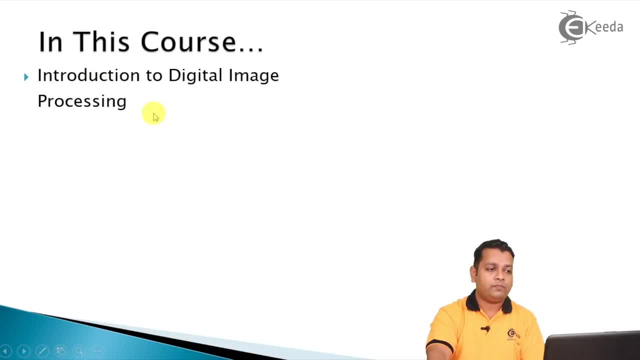 chapter: introduction to digital image processing, The every detail of digital image and processing, along with the application fundamental steps, the components that we are going to see into this first topic, that is, the introduction to digital image processing. This particular chapter will followed by the second chapter, that is, digital image fundamentals. 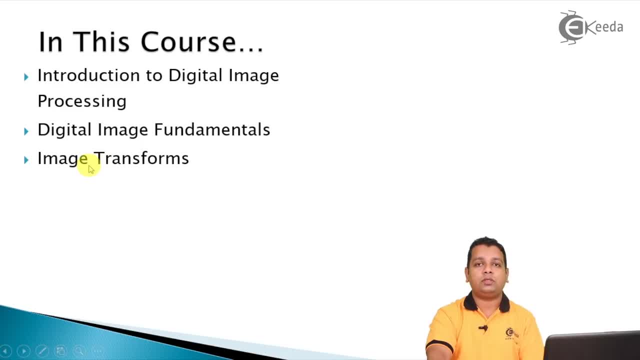 After that we have the different image transforms which will be having the mathematical interpretation. Next to that we have the image enhancement, the improvement of information in the spatial domain, also the image enhancement into the frequency domain. We have image restoration here, the image enhancement into the spatial and frequency domain, and 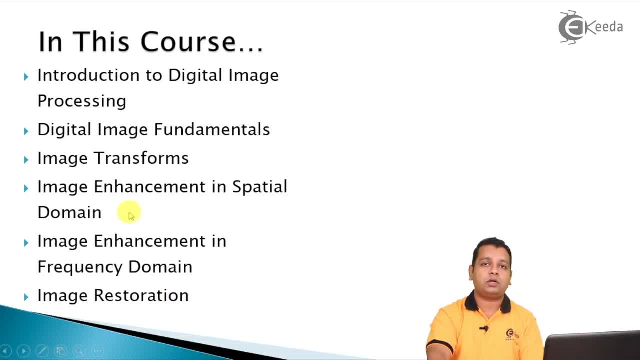 image restoration. all are having the same motto but the different procedures, different types To work on to the improvement of pictorial information after image restoration. we have the color image processing, right from the first chapter to this particular chapter. we have the binary images and the grayscale images address for such operations. and here we start. 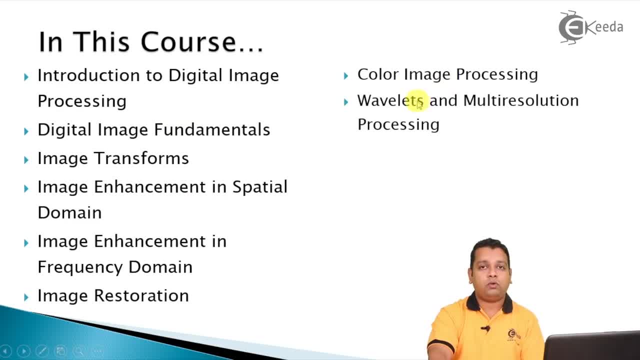 with exactly the color image processing. it will be followed by the very popular and the potential tools, that is, wavelets and multi resolution processing. here the resolution is at multiple level. We are going to have a very potential tool into the applications of the digital image processing. 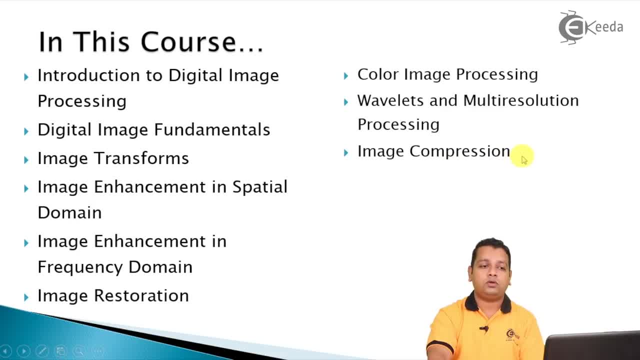 Further we have the image compression, where we are going to minimize the memory requirement to store and to transmit the image from one place to another place, along with some morphological image processing. after image compression and image segmentation, we have further. we have representation and description of image.